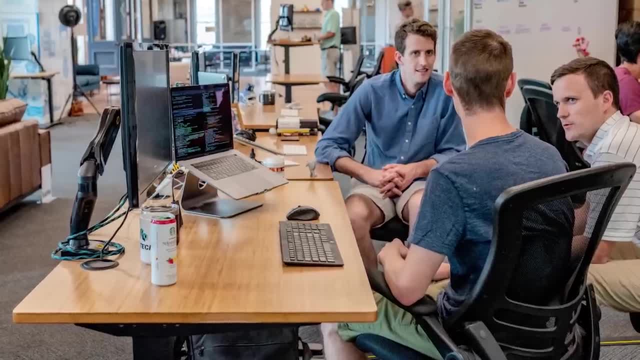 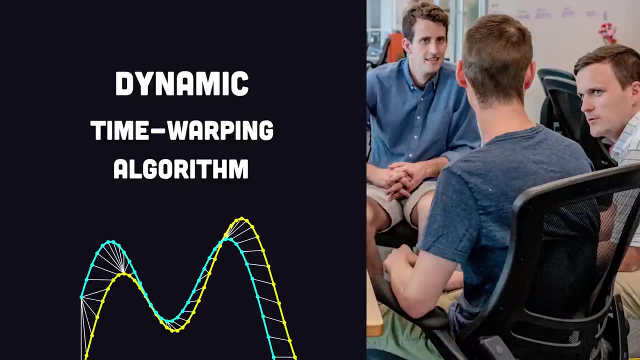 Red green refactor. Imagine you're sitting in a technical interview for an entry-level web developer job and they ask you to implement a dynamic time-warping algorithm to measure the similarity between two sequences and logarithmic time, Instead of freaking out and wondering what. 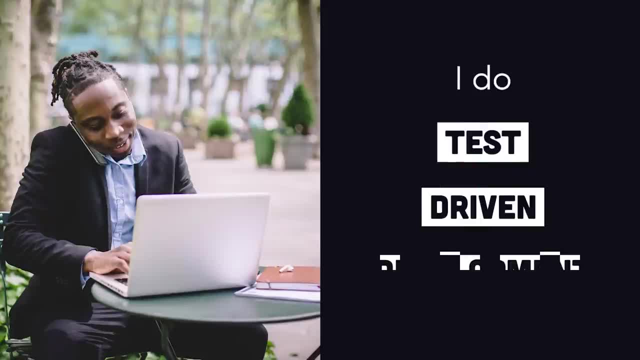 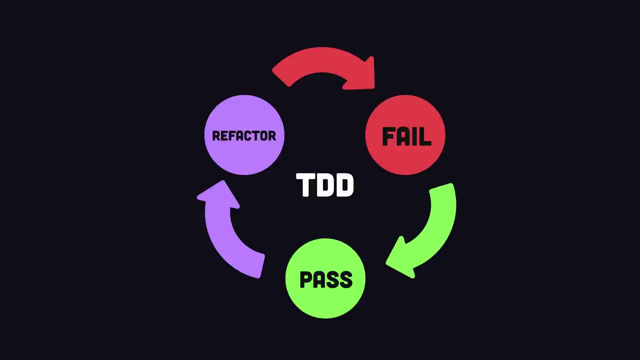 this has to do with jQuery. you can just say: no problem, let me write a few test cases for that first. Not only will that buy you some time, but it also makes you look like you know what you're doing. Test-driven development is a technique where you describe the behavior of your code. 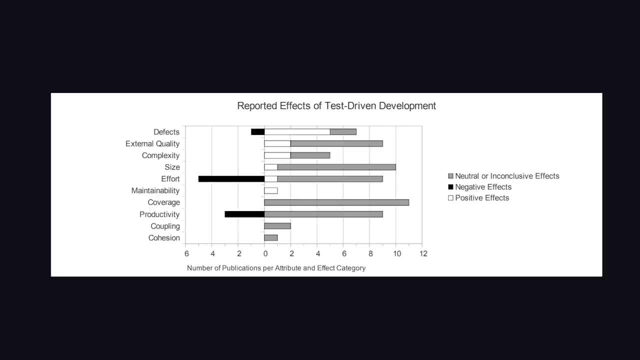 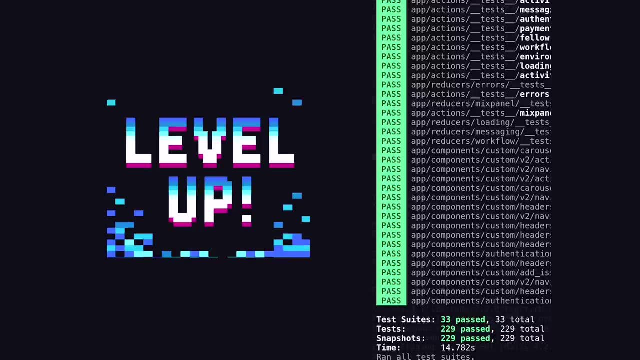 before you go and implement it. If you trust the science, testing will help reduce bugs and improve the maintainability of your code base in the long run. And if you're new to programming, knowing how to test your code is one of the most powerful ways to level up as a developer, Not only. 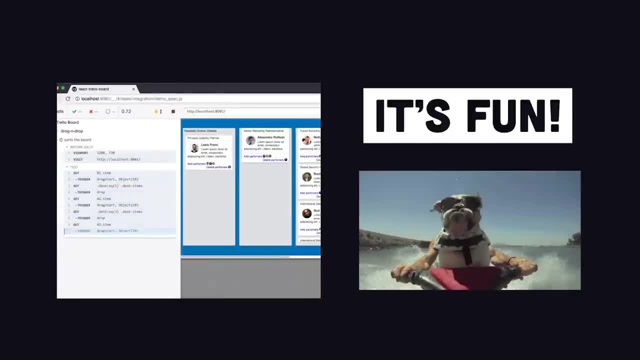 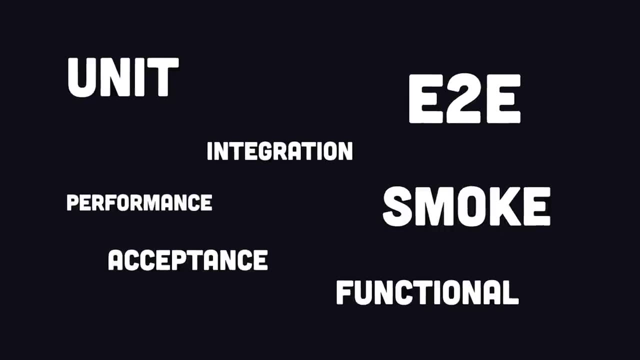 is it fun, but it will also teach you about your code in unexpected ways and make you much better at debugging it. Today's video will teach you everything you need to know to get started with software testing as a developer. We'll talk about a bunch of different testing strategies from a 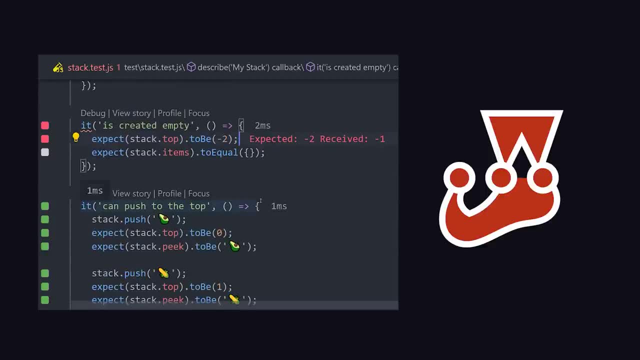 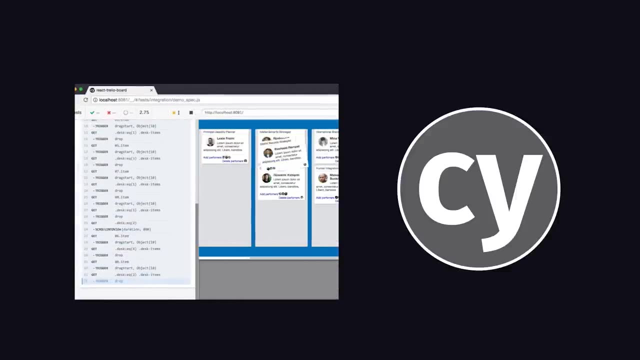 high level, then take a hands-on approach by implementing unit tests from scratch with Jest, and we'll also look at end-to-end testing with a tool called Cypress. But most importantly, by the end of the video you'll learn why testing is valuable and how to make the decision about. 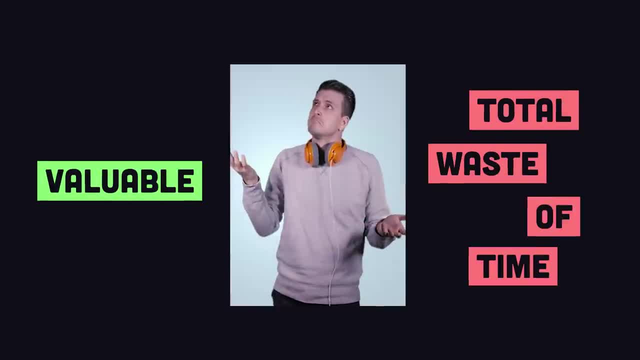 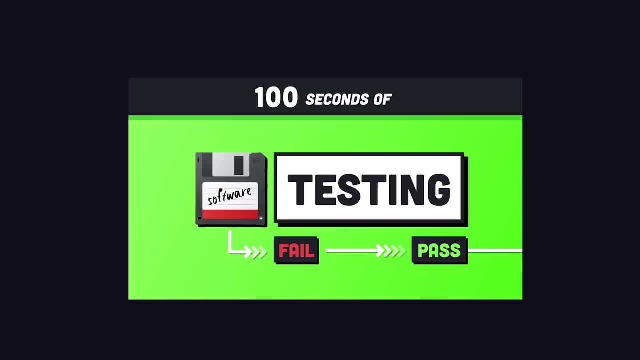 whether or not you should test something, because it's a practice that walks a very fine line between being valuable and a complete waste of time. Before we get started, make sure to hit the like button and subscribe. In the last video, I explained how software testing works, but if you 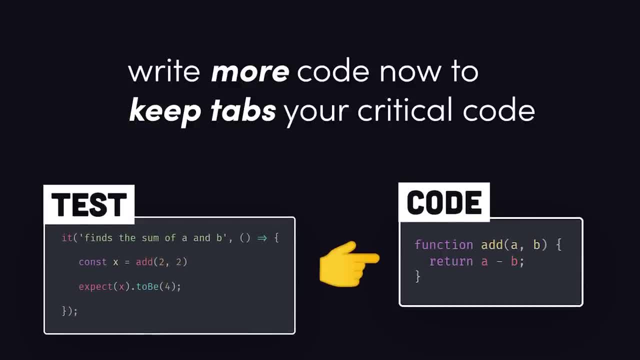 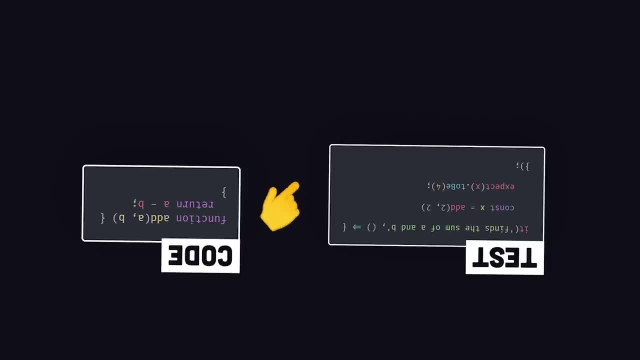 missed it. automated testing is basically just a way to write code that describes your requirements and validates your main application code. Now, most developers I know, and myself included, generally don't start writing tests until we have a working feature, Or maybe we just don't write any tests at all, And that's especially true with 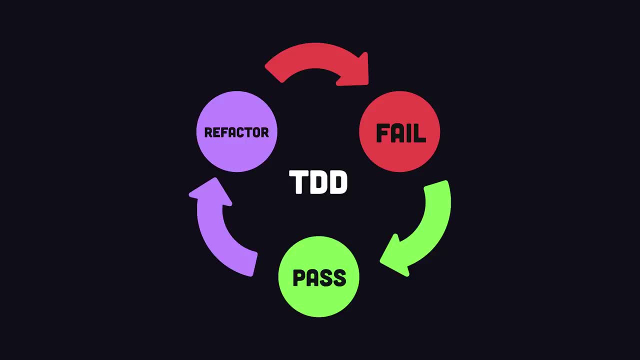 front-end development because UI requirements tend to change frequently. But if you follow the principle of test-driven development, you'll write your test before you implement your actual code. And a common mantra is red-green refactor, which means you write a failing test first, red, then 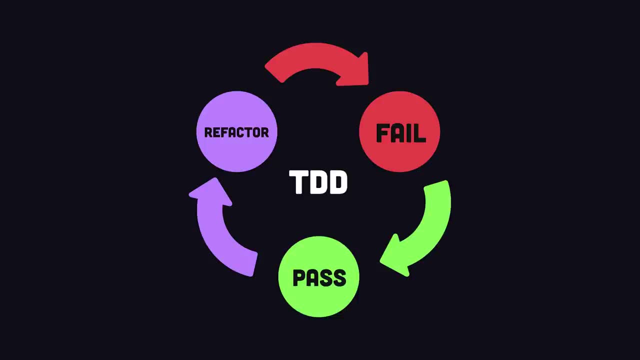 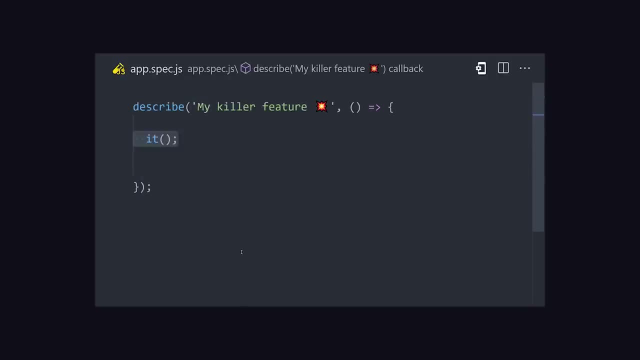 you write some code to get it passing green. then you go back and optimize or refactor the code. It's not always practical to do this, but if you have a project with very clear requirements, you might find that TDD actually improves your productivity. Now let's take a look at a bunch of different testing. 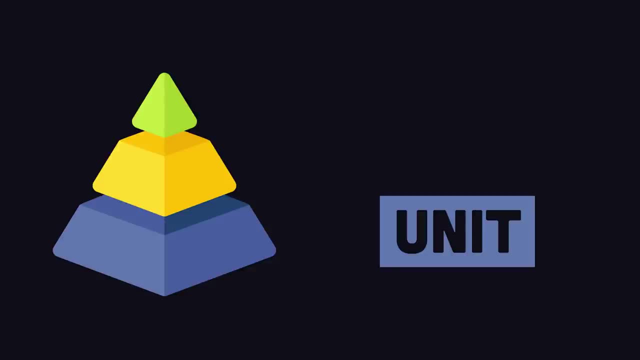 strategies and see how they add value to a code base. At the lowest level we have unit testing, where the goal is to validate the behavior of individual functions, methods or just units of code. We'll get hands-on with unit testing in just a minute. The next level up is integration. 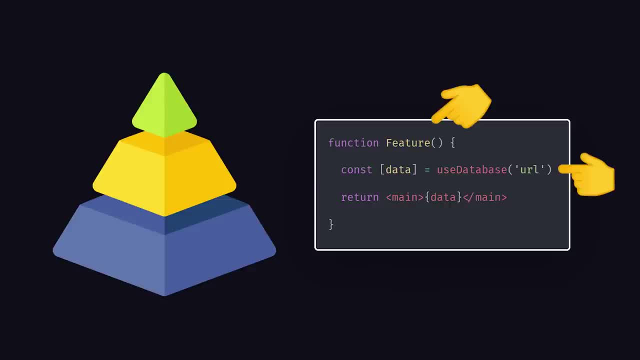 testing, which involves testing multiple units of code together. For example, you might have a React component and a hook to fetch something from a database. You can unit test each of these individually, but then you have to do it in a different way. So if you have a project, that's. 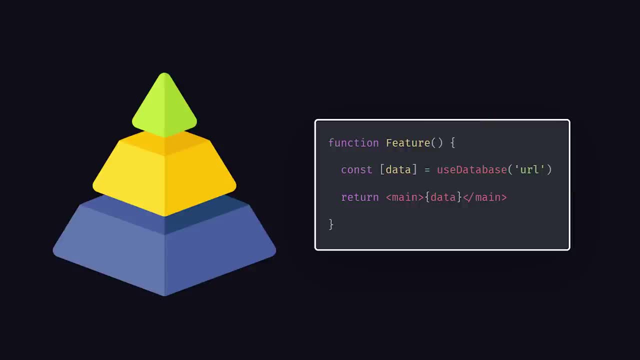 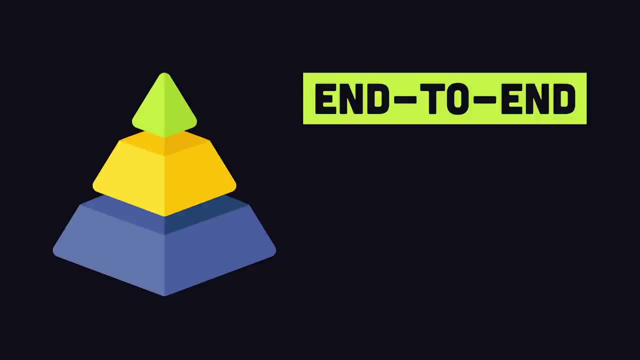 run on a database. you can use the integration test to see how well they work together, Like: is the component actually able to use the hook to get the data that it needs for the UI? From there we have end-to-end testing, which runs your app in a simulated environment, and 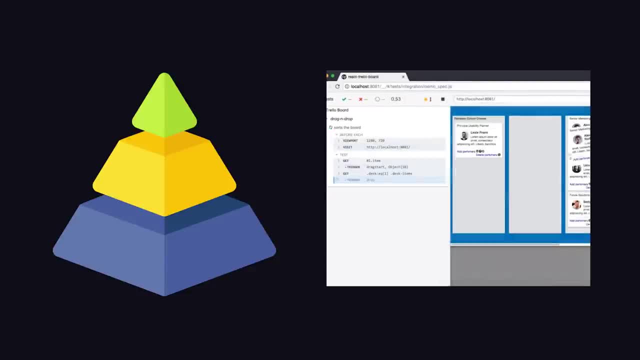 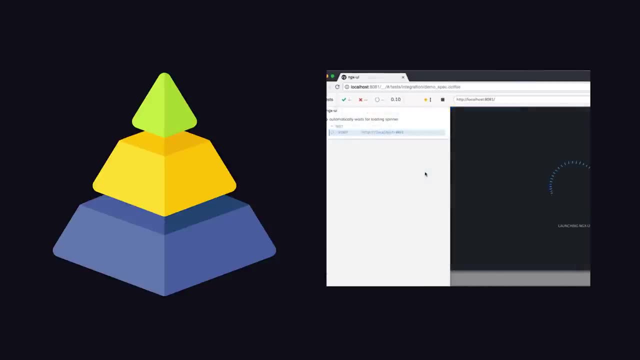 attempts to emulate actual user behavior. There's a really awesome tool called Cypress that has a browser-based test runner that allows you to program tests where users click on buttons, fill out forms, then assert that the actual changes to the DOM or the UI are valid. 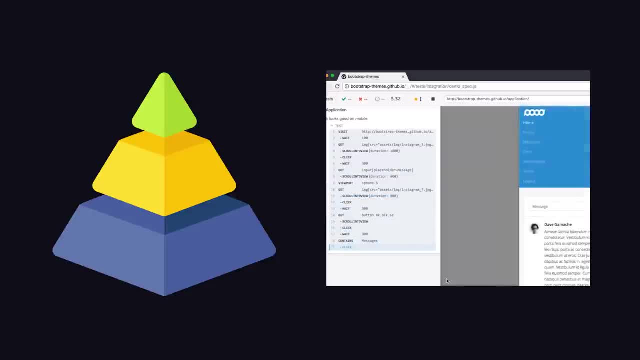 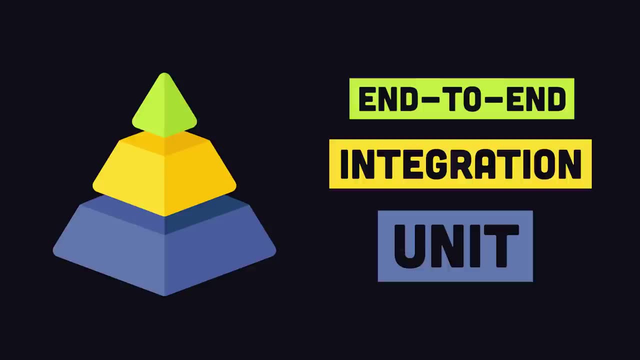 Personally, I find end-to-end tests to be the most valuable ones, so make sure to stay tuned until the end of this video to see Cypress in action. In my opinion, these three testing strategies are the most important ones to know, but there are a lot of other terms that get thrown out there that you may want to be familiar with. 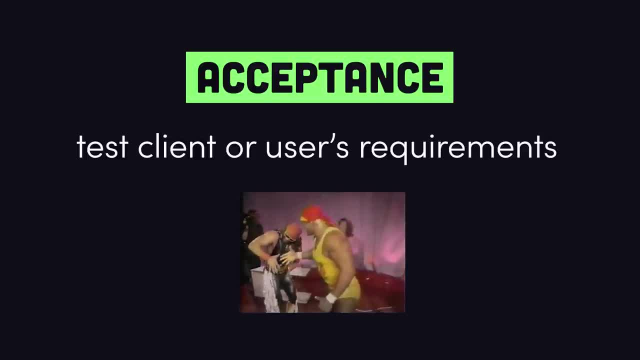 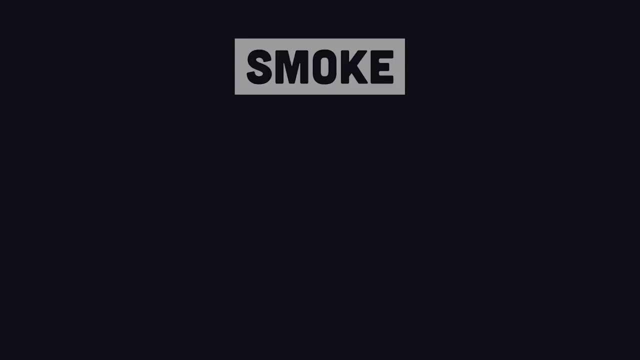 Acceptance testing is a form of testing that makes sure that the software meets all of the client's requirements. Then you have system testing to ensure that everything works on actual servers or hardware. Then you have things like sanity or smoke tests. On a large application. you may have thousands of tests to run and this can actually take a. 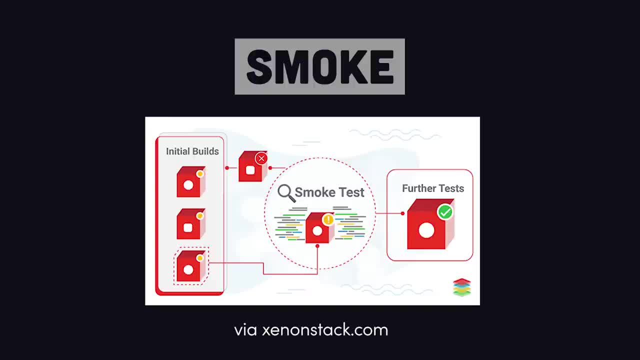 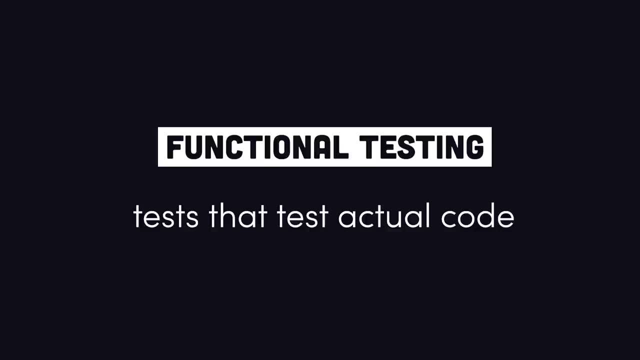 long time. A smoke test runs a few of the most important tests. first, to make sure the app isn't on fire, before proceeding with the rest of the test suite. Now, at this point we've only looked at functional testing, but there are also 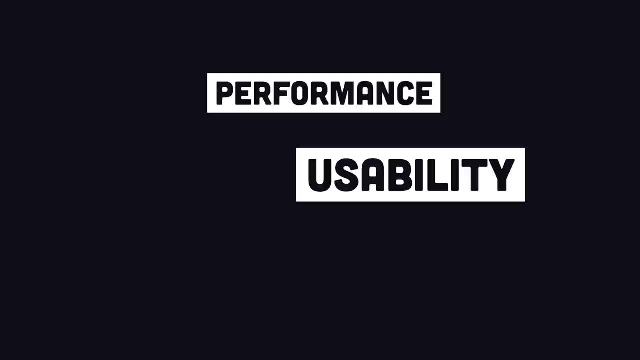 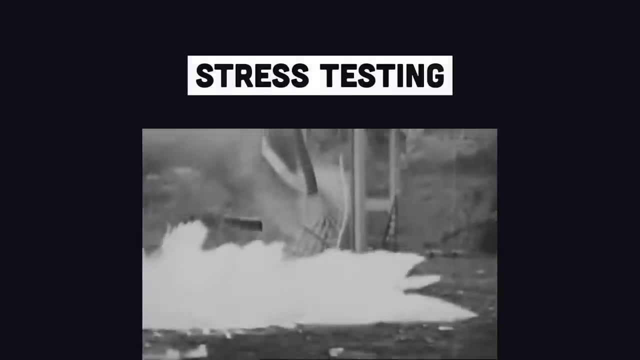 non-functional tests for things like performance, usability and security. You'll often hear terms like stress testing or failover testing, which are used to test the capabilities of the infrastructure as opposed to the code itself. Now that you know what all this fancy testing jargon means, let's get our hands dirty in. 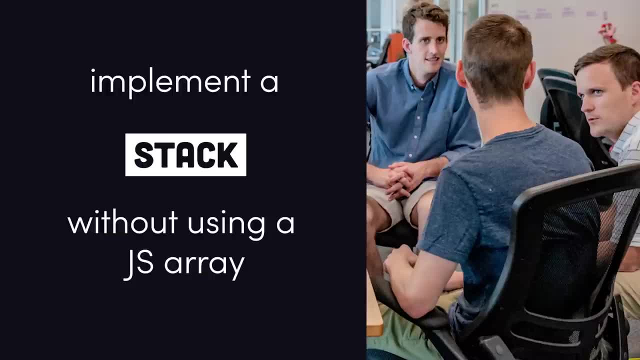 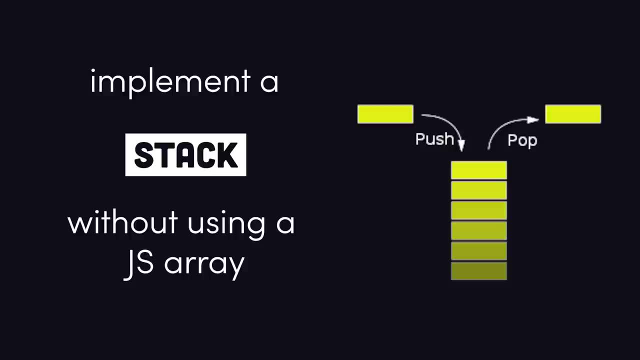 JavaScript by pretending that we're in a system that's not working. We're required to implement a stack data structure where the last item in is the first item out. It's very similar to an array, but we have to implement it without using a JavaScript array. 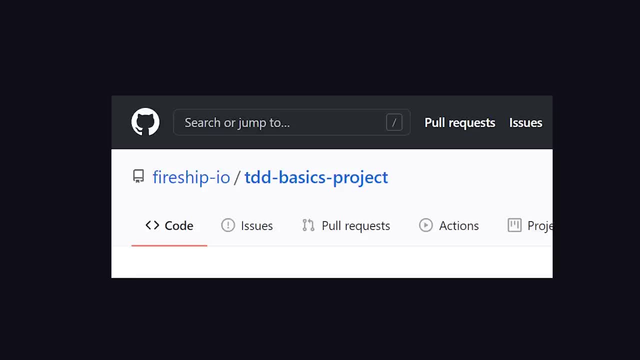 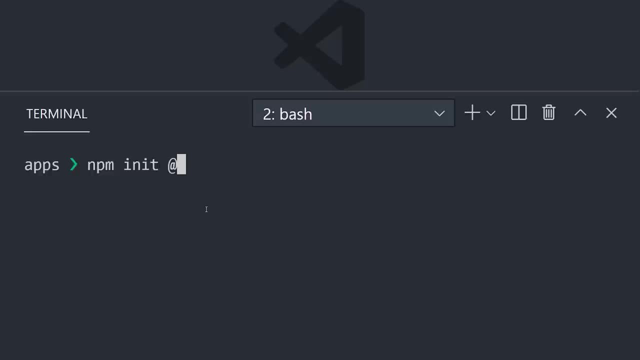 Now, before we can start, we need to initialize a project, and keep in mind that you can find the source code for this on GitHub. I'm using Vite by running the npm init vitejs slash app command, then selecting the vanilla JavaScript option. That gives us a simple project to get started in. 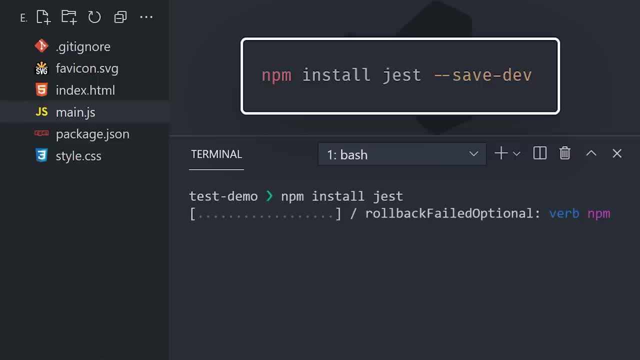 then I'll add the javascript to the project. and then I'll add the javascript to the project. I'll also add a test testing framework to it by running npm install jest, which itself will be looking for any files in your project that end in testjs. 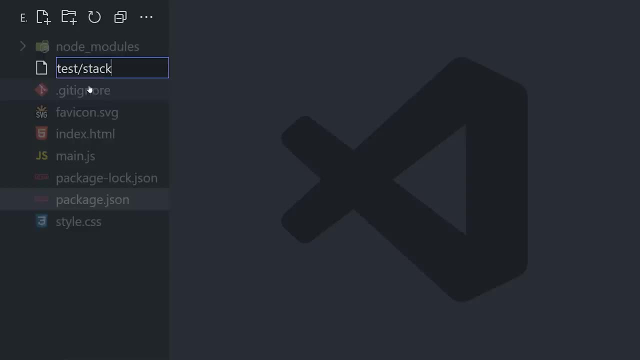 Let's go ahead and create a test directory, then add a testing file to it. To keep things simple, I'm going to implement our code and also test it in the stacktestjs file. Now, to run the code in this file, we need to execute the jest test runner. 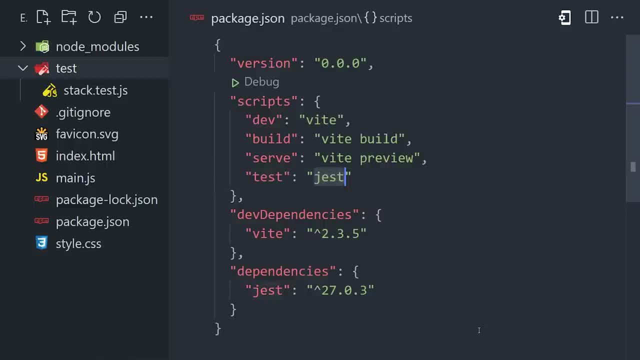 We can do that by going to our packagejson and setting up a new npm script called test to the jest command. In addition, I'll add the watchall command to have jest watch our code in the background and rerun the test any time it changes, and also the verbose flag to add some extra output to the terminal. 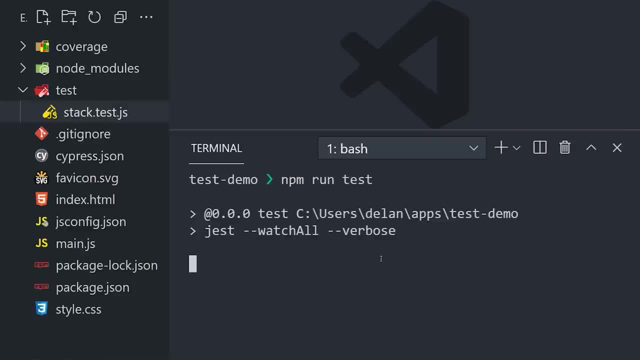 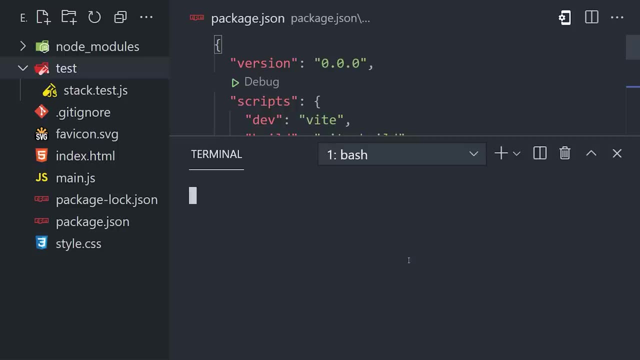 Go ahead and run npm test from the command line and you should get your first failing test, because it's detecting that file, but we haven't actually written any code there yet. One other optional but highly recommended thing we can do here is add types to the project. 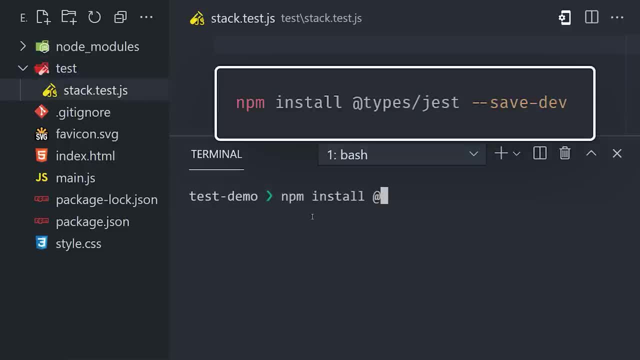 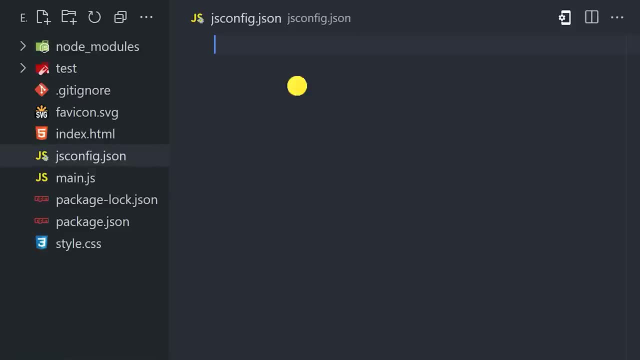 to give us IntelliSense for all the matchers built into jest. Install the types using npm test. then create a jsconfigjson file that has a type acquisition property for jest. This will allow VS Code to provide IntelliSense for everything built into jest, making your life way easier. 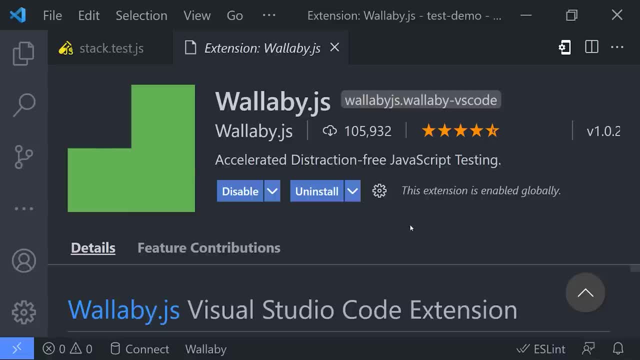 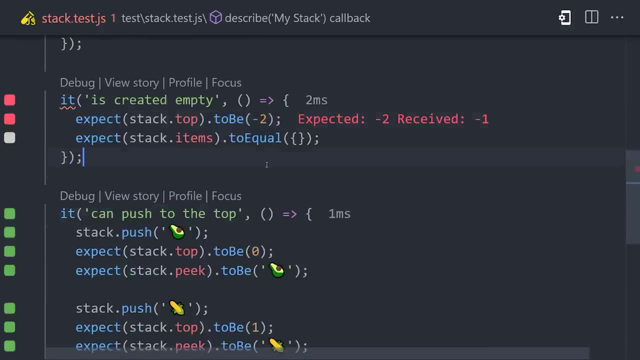 One other random pro tip I'll throw out. there is that you may also want to install the wallaby plugin. It's a paid VS Code extension with a free trial, but it will tell you whether or not your tests are passing directly in the editor. 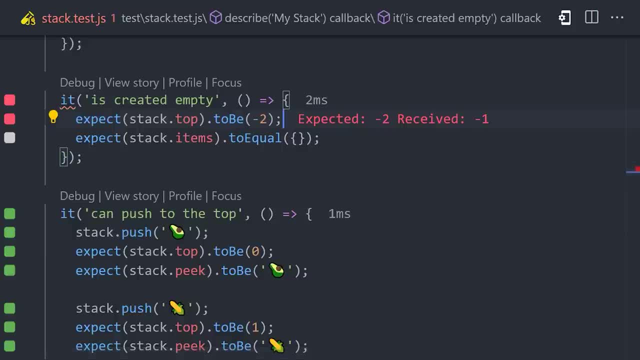 without having to look at the terminal, and that can give you a really nice productivity boost. I'm going to use the terminal on my PC, but I'm going to use it on my PC, so I'm going to use it on my PC. 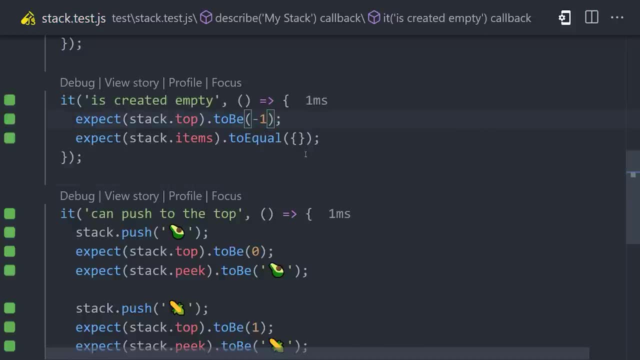 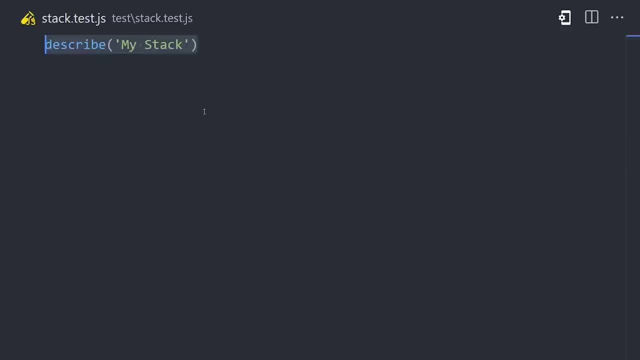 I'm going to use the terminal on this video, but Wallaby was nice enough to provide us with a discount, so feel free to check that out in the description below. And now we're ready to proceed with our interview. The first thing I'll do is use the describe function to describe the thing it is that I'm testing. 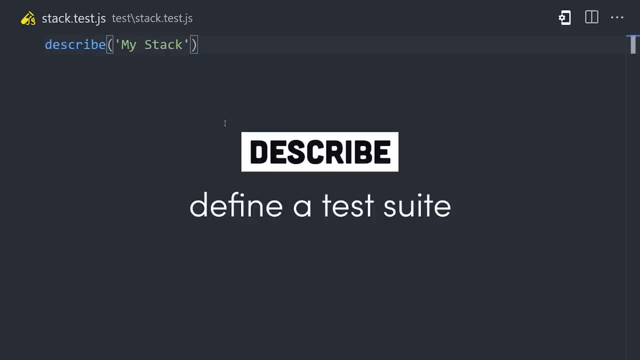 which in this case is the stack. It takes a callback function as the second argument, inside of which we can define multiple individual tests by using the test function or it, both of which do the exact same thing. We'll create a very simple test suite here with only three requirements. 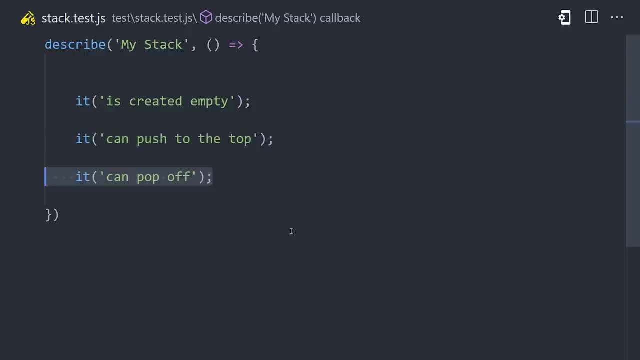 It is created empty, that it can push items to the top and it can also pop or remove items from the top. At this point, if we go ahead and save the file, we should get a failing test suite because we've only described our requirements and haven't actually implemented any testing code yet. 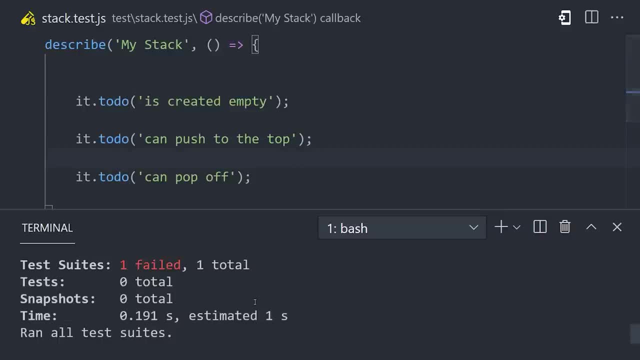 In some cases, you may want to hold off on the test implementation, in which case you can use the to do method to make the test pass. while you figure things out, Now let's go ahead and implement our first test. The main goal of the first test is to ensure that our stack can be instantiated with a valid state. 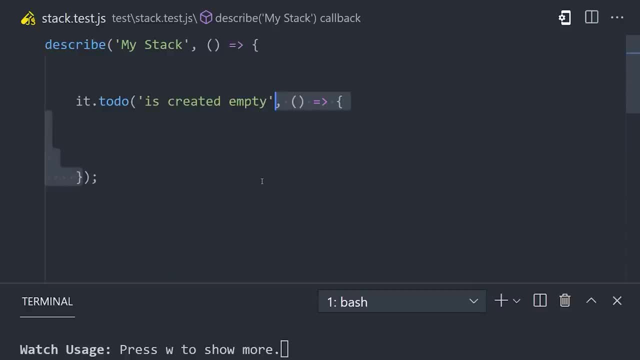 The main goal of the first test is to ensure that our stack can be instantiated with a valid state. Let's go ahead and instantiate a class that doesn't exist to represent the object that we want to test. From there, we'll use expect to write an expectation to make sure that our code does what is expected. 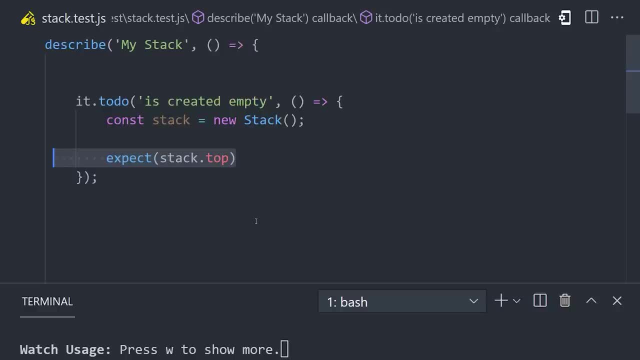 It should have a top property that represents the index of the item at the top of the stack, Because it's empty when it's first created, the value should be negative. one To be is a matcher that will test the actual value to the correct value. 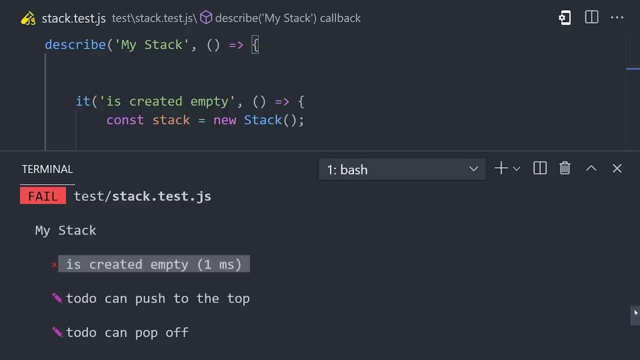 Now here's where test-driven development starts to get really cool. Go ahead and save the file and you'll notice that we get a failing test. If we look at the output closely, it'll tell us exactly which line of code failed and why. 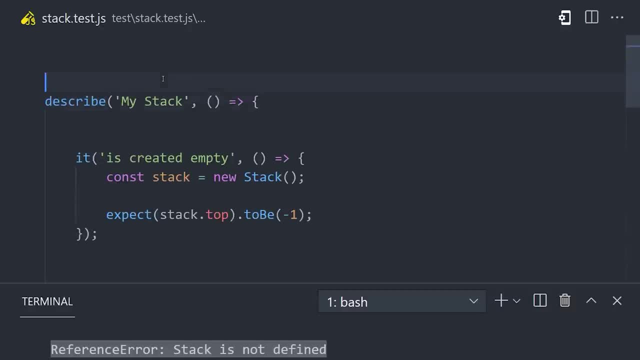 It says: reference error: stack is not defined. We can use that feedback as a starting point to start implementing our code. To address the error, we'll first need to define a class called stack. Go ahead and define it, then save the file. 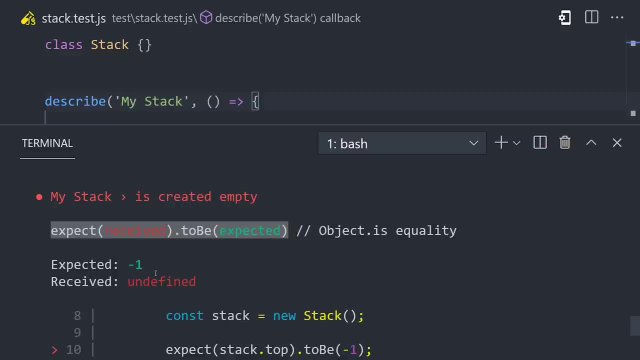 Then you'll notice that we still get a failing test, but this time it goes down to the expectation, telling us that it expected negative one but received undefined as the return value. To address that issue, we need to add a constructor to the class. 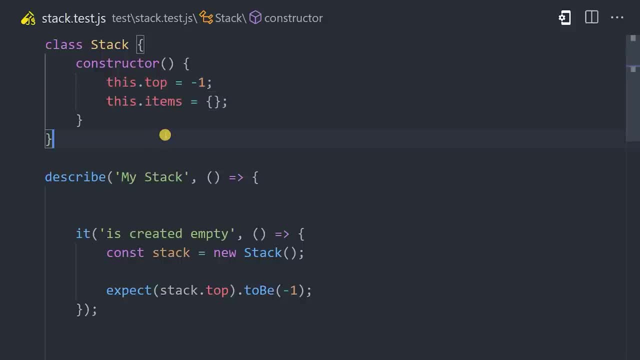 to initialize it with the proper data. Let's give it a top value of zero, and then we'll also define an items property here to represent the stack itself as an empty object, Because, remember, we're not allowed to use arrays in this problem. 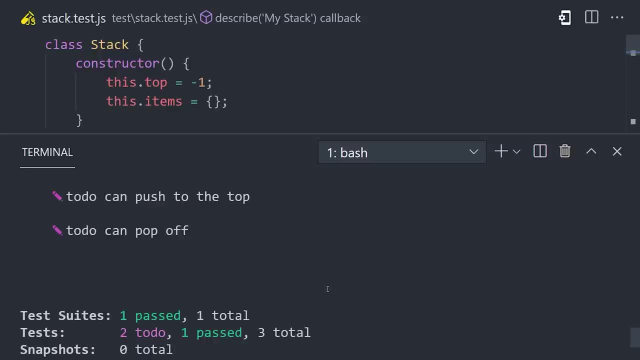 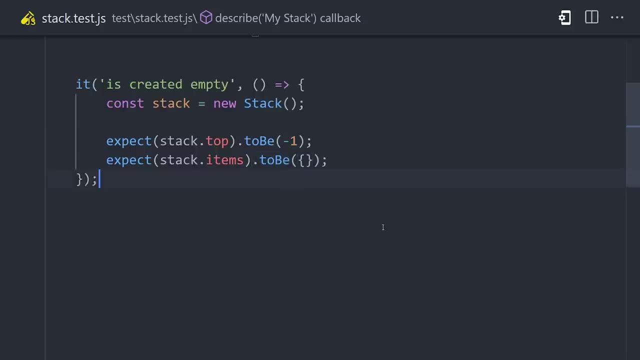 Go ahead and save the file, and now we finally get a passing test. You can also add multiple expectations to a single test. Let's go ahead and test the stack items property to make sure that it's an empty object, But when we do that, you'll notice that it's empty. 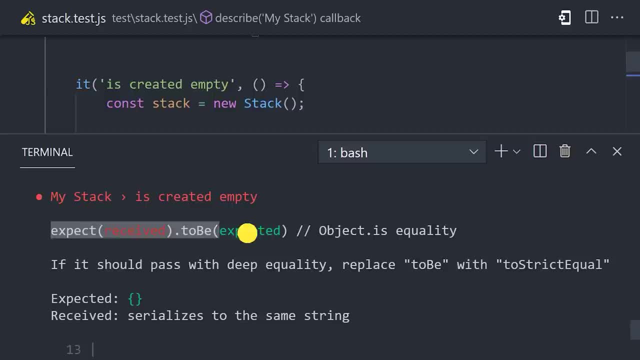 You'll notice that we now get a failing test, even though we're definitely comparing an empty object to an empty object, And it's actually not an issue with our implementation but an issue with the test itself. The toB matcher checks for referential equality. 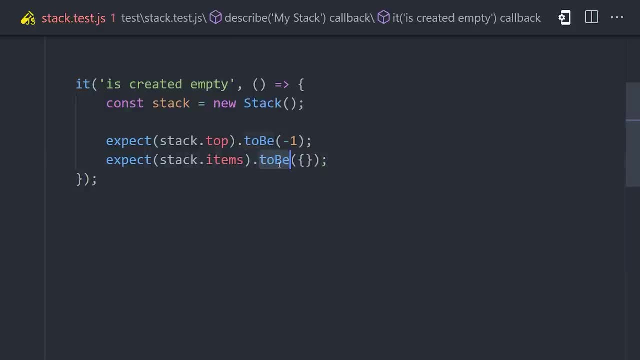 between two objects. In this case, both objects are empty, but they're two different objects in memory, which is causing the test to fail. What we need to do here is use a different matcher. The toEqual matcher would be a better choice. 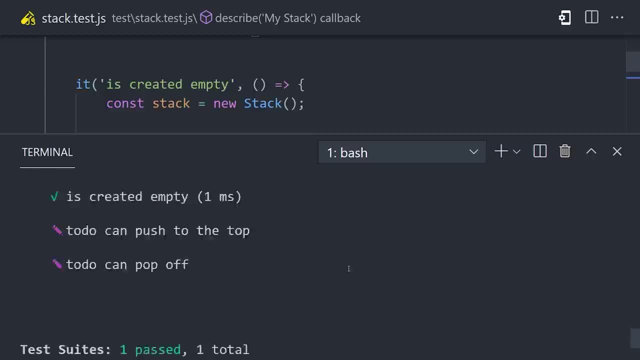 because it checks for value equality instead of the object reference itself. An important takeaway here is that it's not always your main application code that's the problem. It might be a bug in the test itself, and unfortunately we don't write tests for our tests. 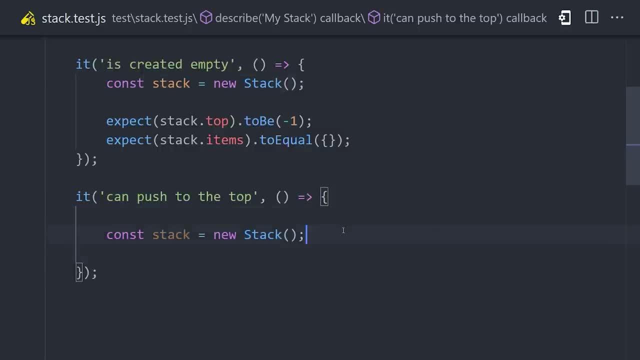 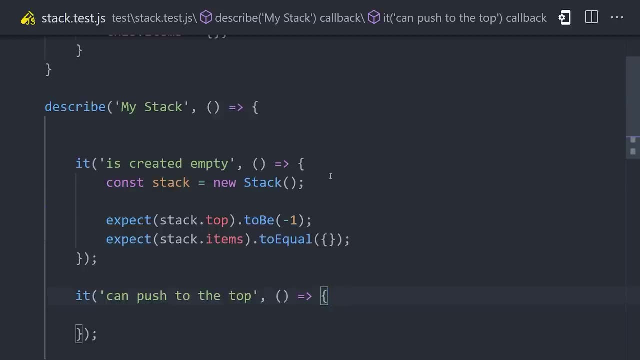 Now let's move on to our second test, to see if a stack can push an item to the top. What you'll notice is that the first thing I'm doing is initializing a new stack, just like we did in the previous test, But there's actually a more efficient way to do this. 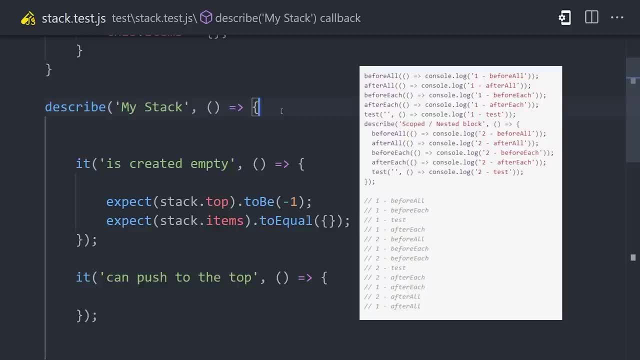 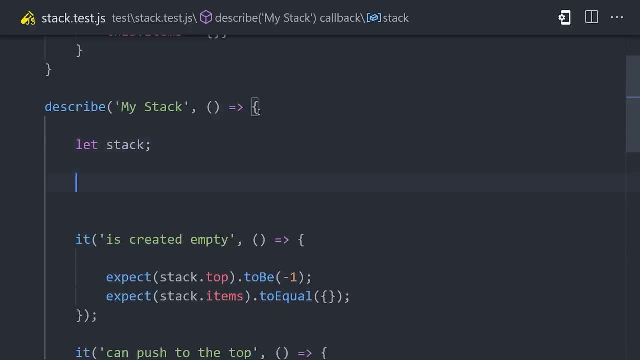 Jest has a set of helper functions for setup and teardown. These are really useful because code duplication can get really bad inside of a test suite. For example, we might set up a global variable for the stack, then use the beforeEach hook to reinitialize it. 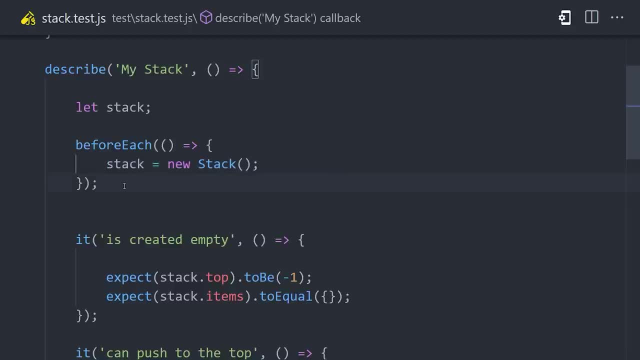 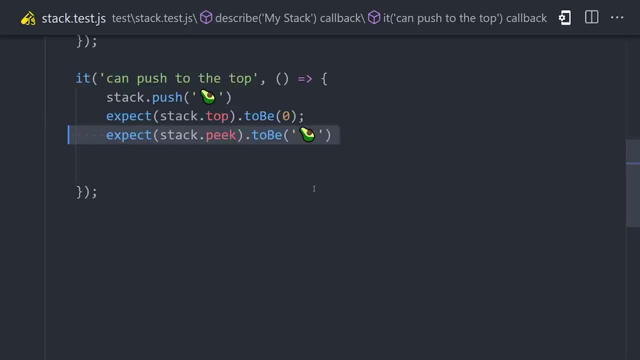 before each new test. That'll give us an empty object to work with before each test, so we don't have to set it up manually in each one. Now, going into our second test, we'll call the push method with an item and then we'll expect the top value to be incremented by one. 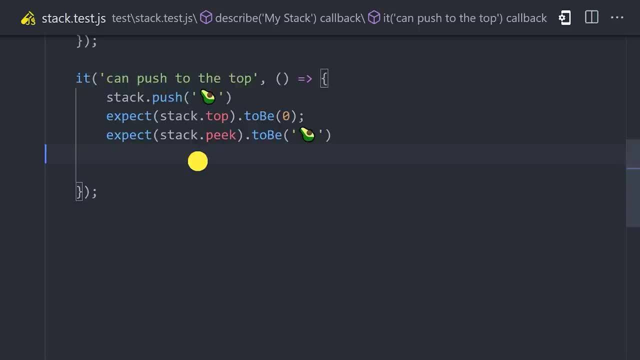 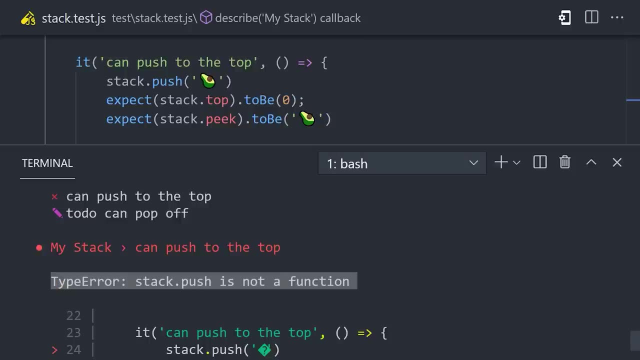 and we'll add a peak property to get the top of the stack and we'll expect that value to equal the value that we just pushed to it. That'll give us a failing test and then we can once again go into our source code and start implementing. 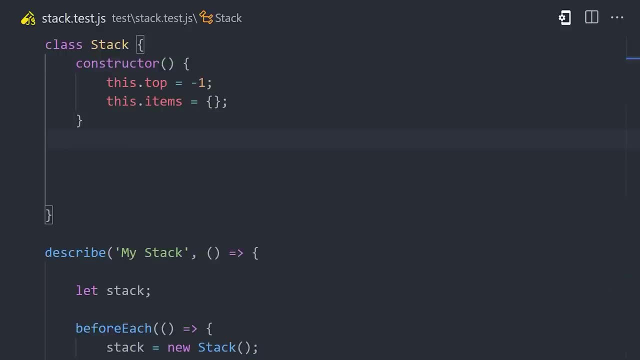 the features needed to get to a passing test. In general, what you'll wanna do here is try to get to a passing test as soon as possible. Once you have that passing test, you can then go back and refactor and look for optimizations to make. 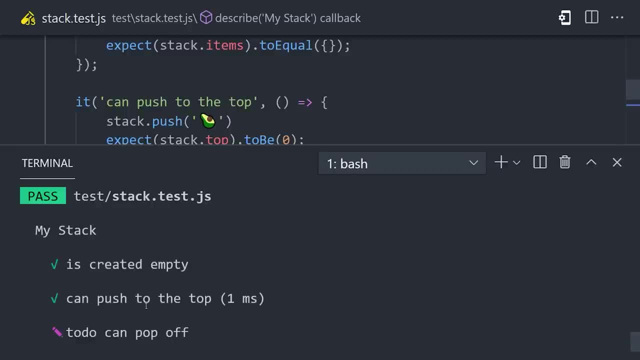 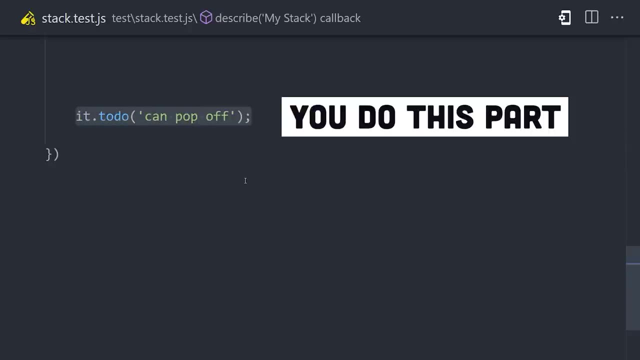 while trying to keep your test in the green. There's just something very psychologically satisfying when you go from a red failing test to a green passing test. My challenge to you is to now implement the final requirement in the test suite. Try to use test-driven development to implement a feature. 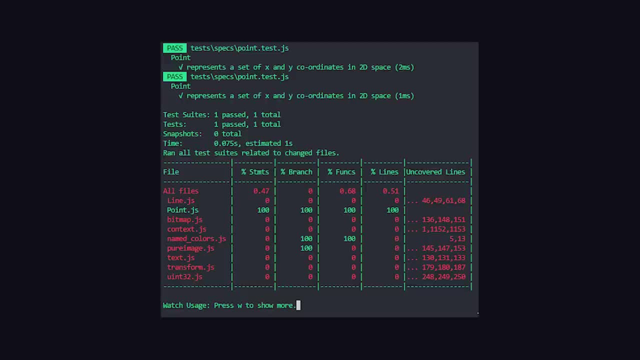 that can pop an item off of the stack. Speaking of psychologically satisfying. another thing you can do is run a code coverage report, which will give you an idea of how well your tests cover your actual source code. Back in the package JSON, add the coverage flag to the just command. rerun it. 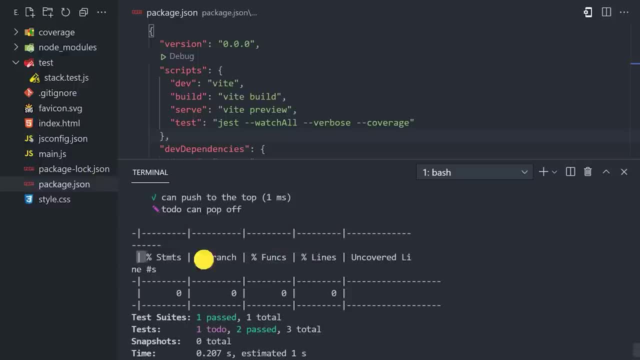 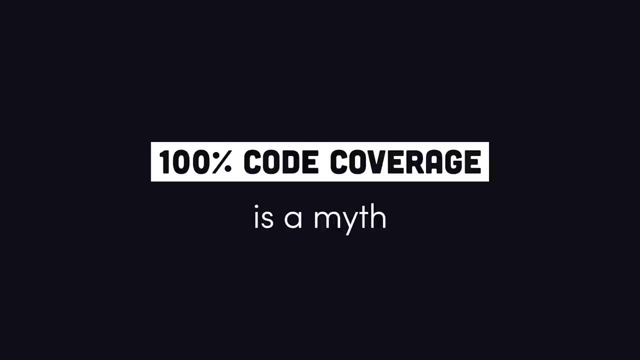 then you'll get this report generated that tells you the percentage of code covered by your test suite. That can be useful at times, but mostly it just gives you a false sense of security. 100% code coverage doesn't mean that you have a good test suite. 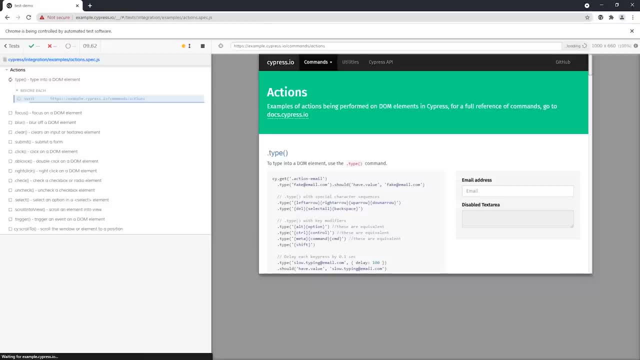 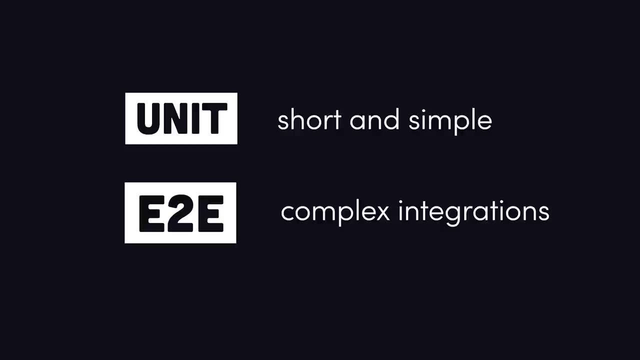 but it may be a good thing to show your product manager, your client. What I wanna show you next is a lot more fun and interesting, and that is end-to-end testing, Unlike a unit test which is designed to be fast and simple. 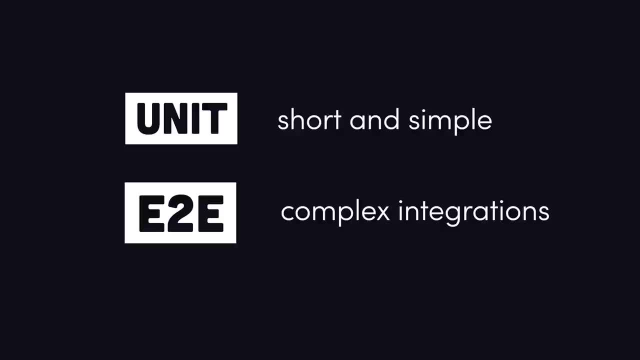 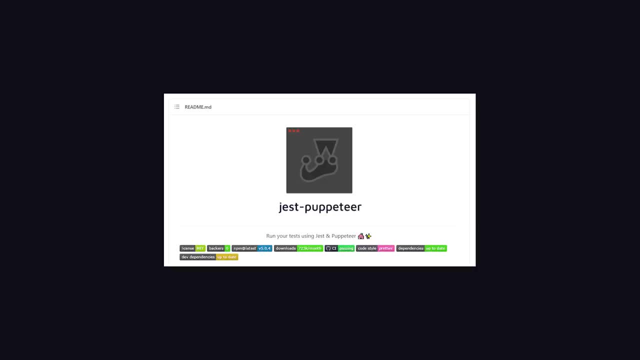 an end-to-end test is very long and complex and takes a while to run, because it simulates actual user behaviors in the browser. We could write our end-to-end test with Jest utilizing the puppeteer package. However, my favorite way to write end-to-end test- 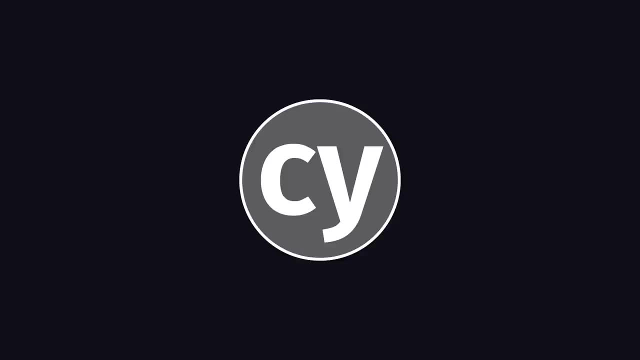 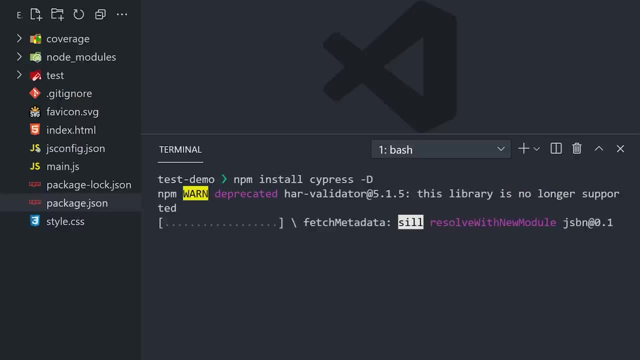 is with a tool called Cypress. Install it by running npm. install cypress, and this will take a few minutes because it's downloading an actual browser that will run your tests in a real-world environment. When the installation is complete, we can go into our package JSON. 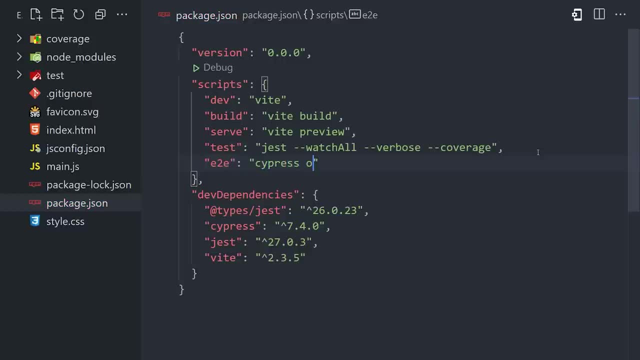 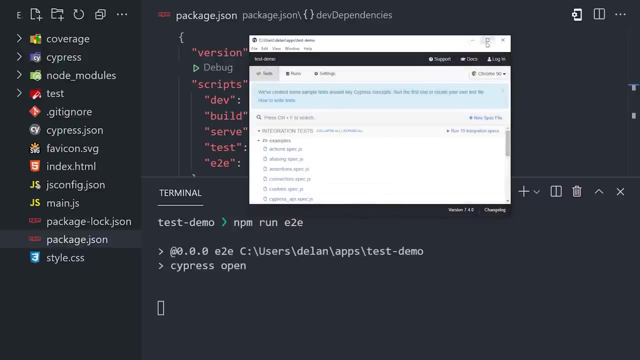 and add an end-to-end script that runs the cypress open command. That should open up the test runner, which comes with a bunch of built-in examples. If you click on the actions example, you'll notice it starts running a test suite by filling out a form, clicking on buttons. 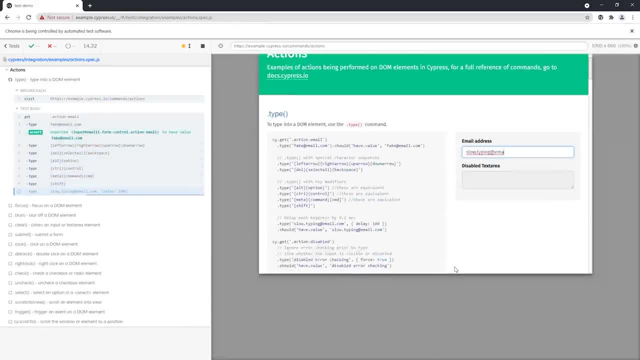 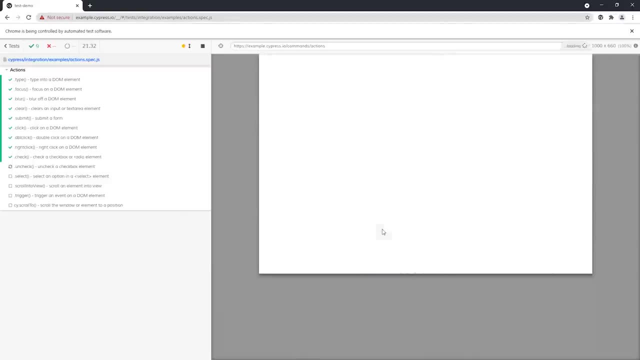 and doing all kinds of other stuff. When I use Cypress for my own projects, I use the Firebase emulator to create a mock database and mock user authentication, which allows me to test my apps efficiently in an environment that is very similar to how they'll look in production.